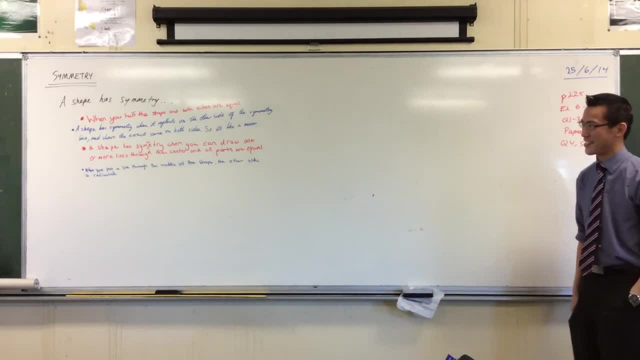 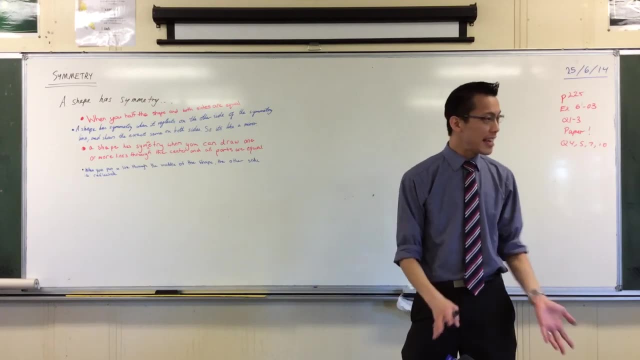 Excellent. Let's have a look at some of these definitions Now. by the way, I think this is really cool- When I was walking around, pretty much no one had exactly the same sentence, Even though you all mostly had a sentence some more helpful than. 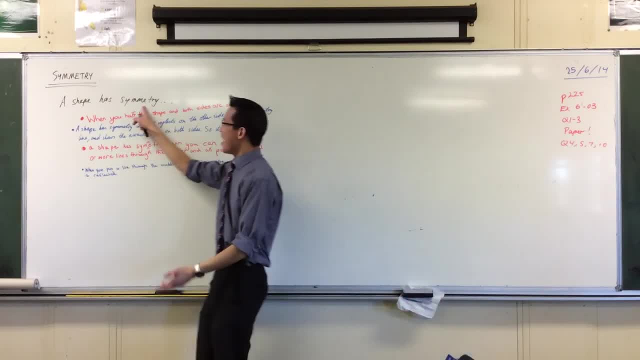 others. But this idea of symmetry it's very common. It's not just common to young people but it's actually a really important idea in the study of beauty. right, They say there's studies actually out there which say that things. 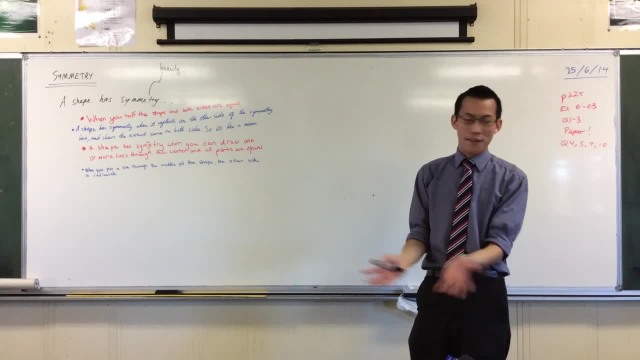 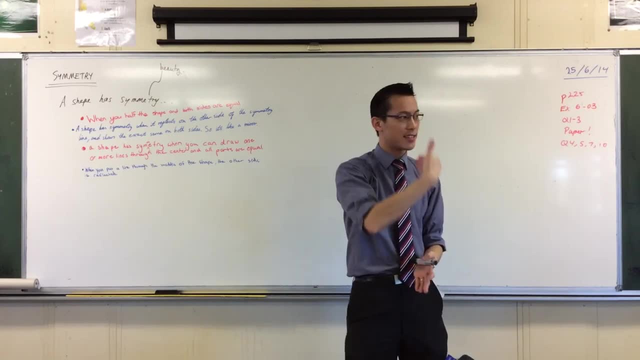 which are symmetrical, are things which we view as beautiful And in fact, you know when you say, oh, someone's really good looking. one of the things, the qualities that they say good looking people have, is that their faces are very. 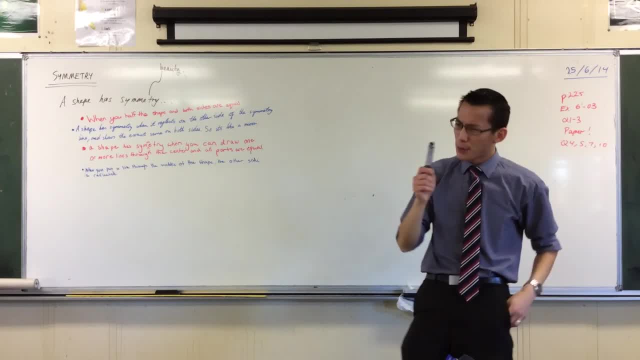 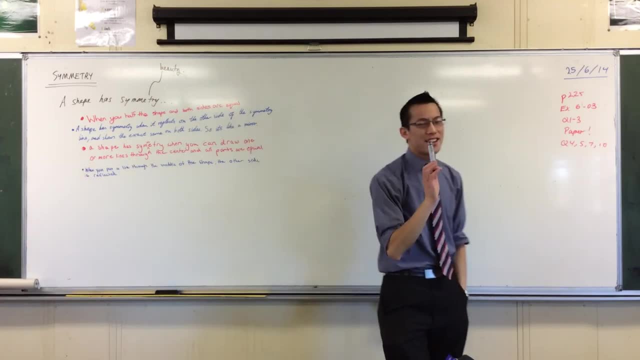 symmetrical, And when a face is not quite symmetrical, we can't put our finger on it, but we say: ah, yeah, it's, yeah, sorry, buddy, You know. so symmetry is a super important idea And it's really really profound. Let's have a look at. 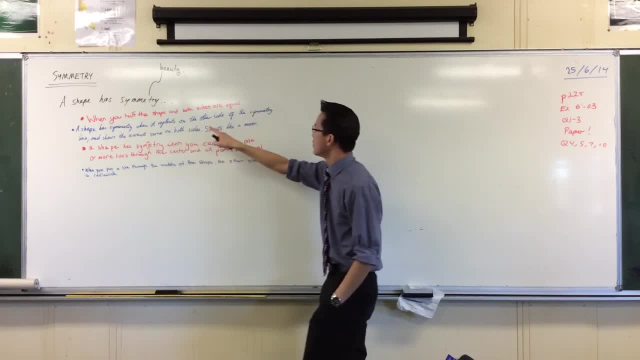 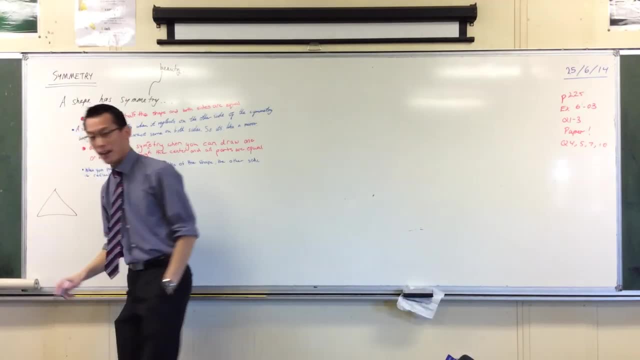 some of these ideas. When you halve the shape and both sides are equal, Hmm, okay. so the idea is: you've got a, you've got a shape like this or something like that, okay, like this. And if you chop it in half, both sides are equal. So if I sliced it like this, then 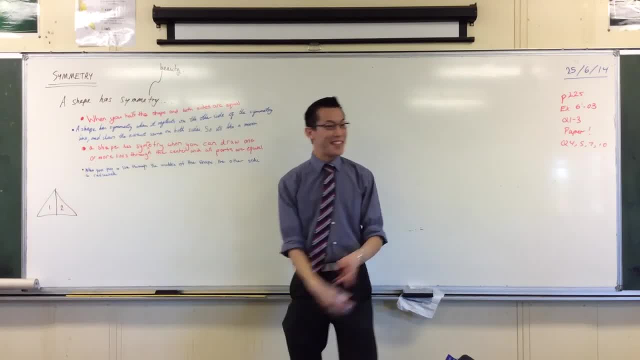 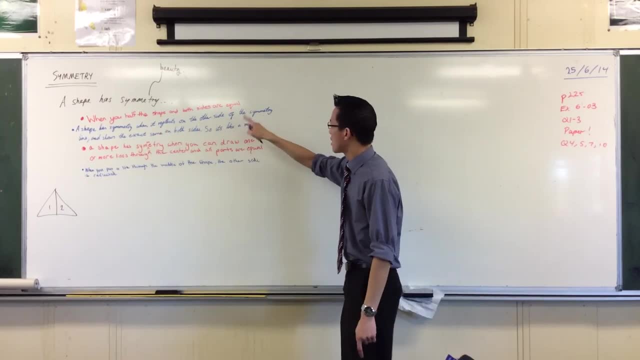 you've got this side and this side and they're kind of well- not on mine, but they're meant to be equal. All right, I think that's a good idea. Let's keep going. A shape has symmetry when it reflects on the other side of the symmetry. 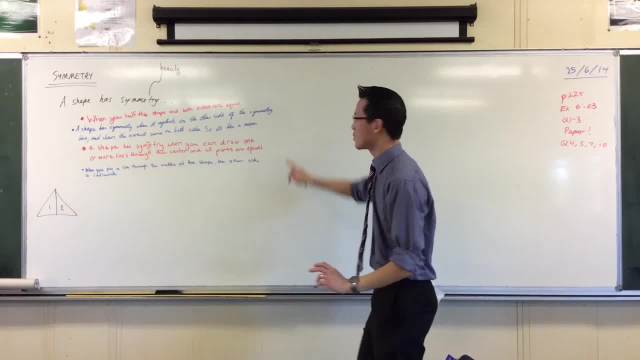 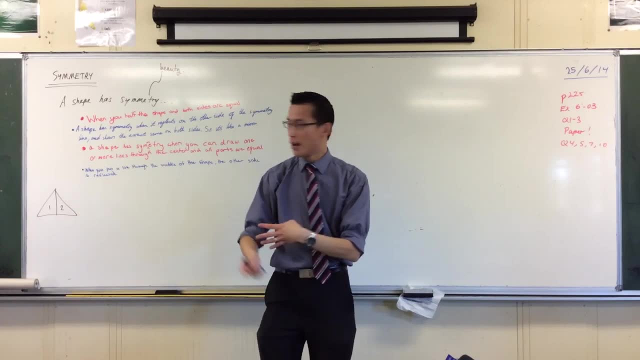 line. Okay, hold on, hold on. Lots of words here. Whose was this one? again? This was yes. well done, Amy. Okay, so if I come back to this diagram, I guess we would call the symmetry line a bit like the line. 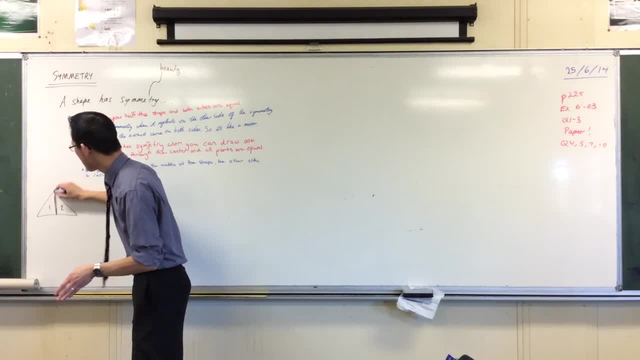 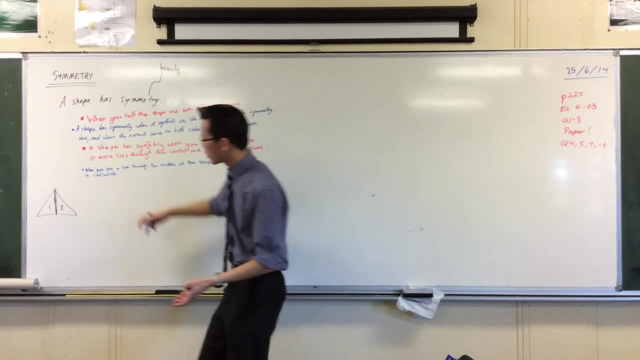 that we use to halve the shape, right, This guy, He seems important, okay, And it reflects on the other side and you get the exact same on both sides. so it's like a mirror, Ah, okay. So it's like. it's like this triangle over here is looking at a mirror and this: 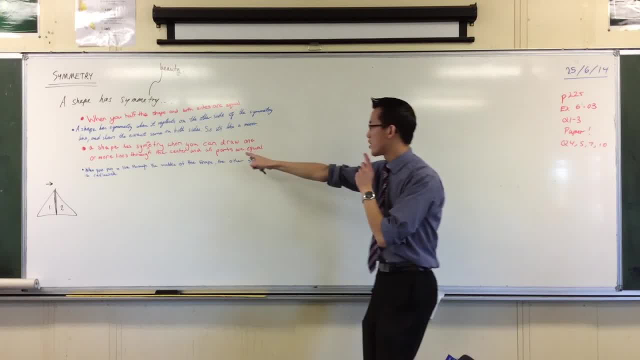 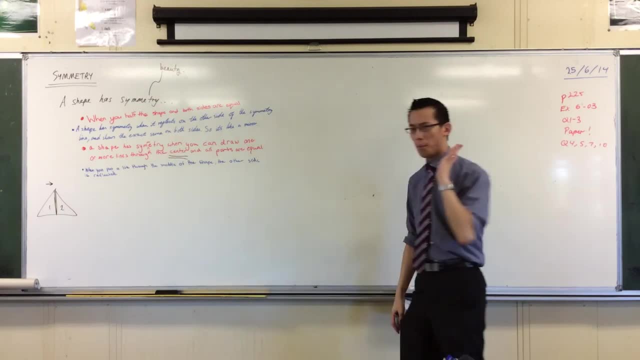 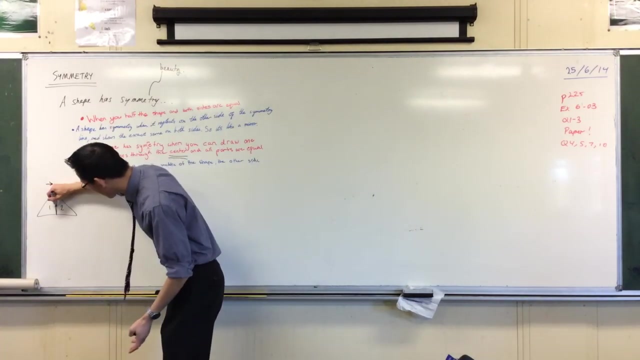 is what the reflection looks like. Okay, cool. A shape has symmetry when you can draw one or more lines through the aha, through the centre, That's a different idea. And all parts are equal. Okay, where would the centre of this shape be? Maybe somewhere like 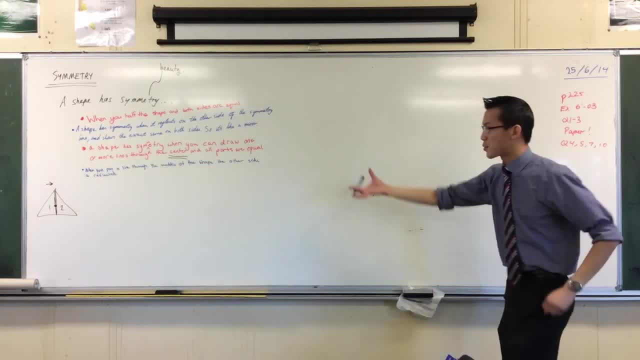 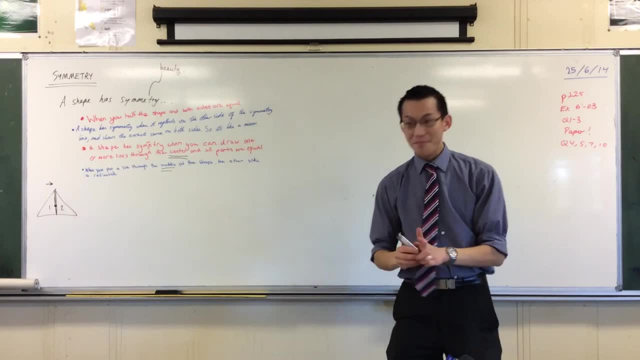 this. Okay, so you've got to draw a line through it. Last one: You put a line through the middle of the shape. Okay, that's again getting the same idea. The other side is reflected. Okay, I think these are all really good. They're all getting at the idea, They're all correct. 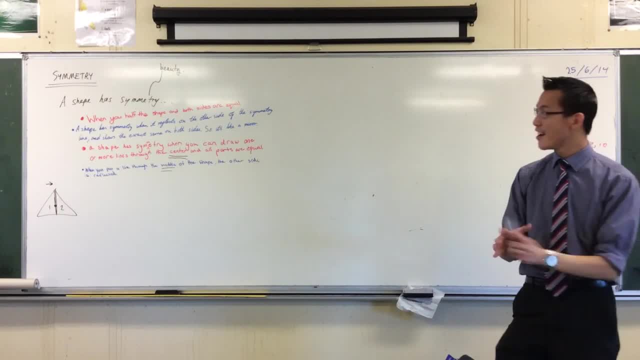 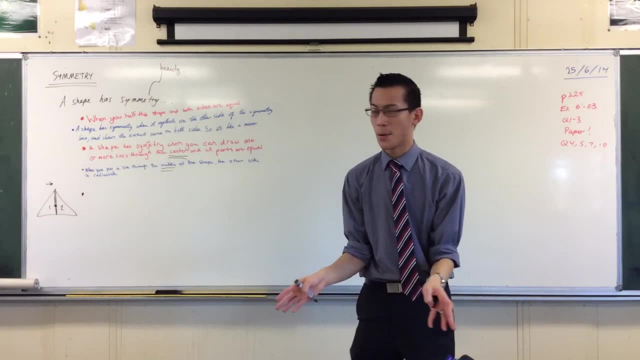 I want to give us a little more detailed definition And I want to connect it to what we looked at over the past couple of days. right, What have we looked at under geometry? What were the first things we looked at? Do you remember? 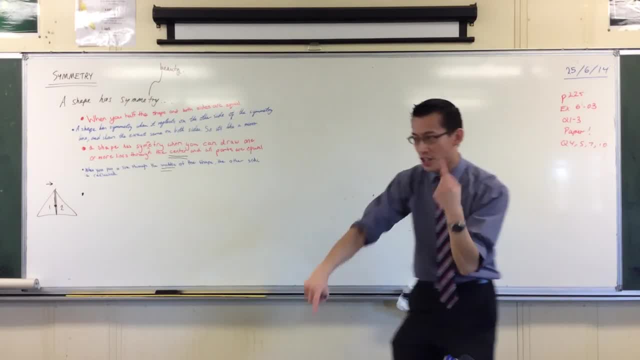 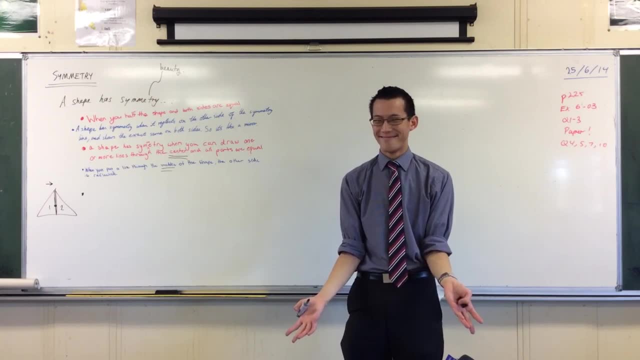 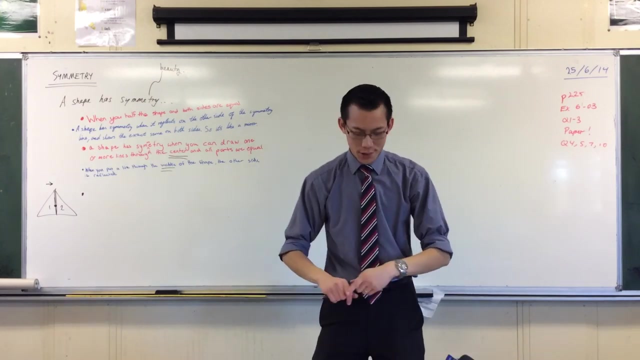 what they're called- Yeah, Yeah, translation and reflection and rotation, And all of those together they're called Long friends, Transformations. That's right, Okay. So I'm going to write a definition for you. that's in terms of those, and I want you to copy it down and we'll discuss. 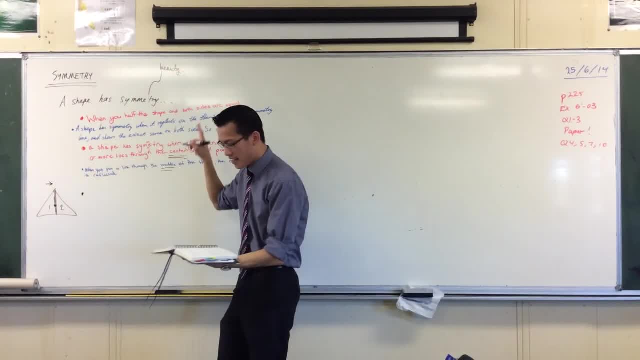 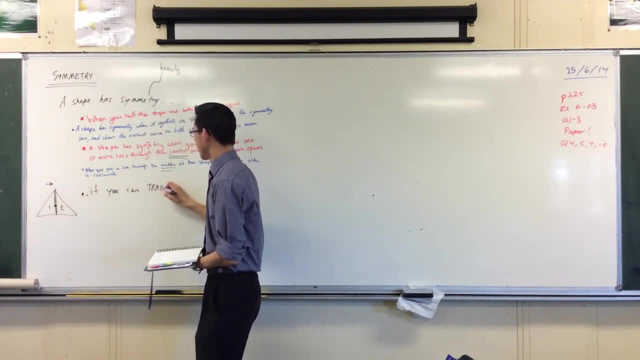 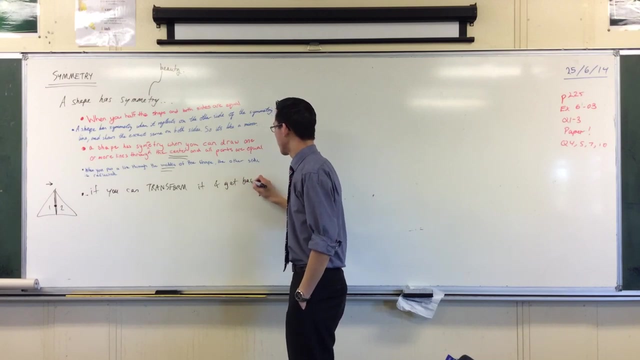 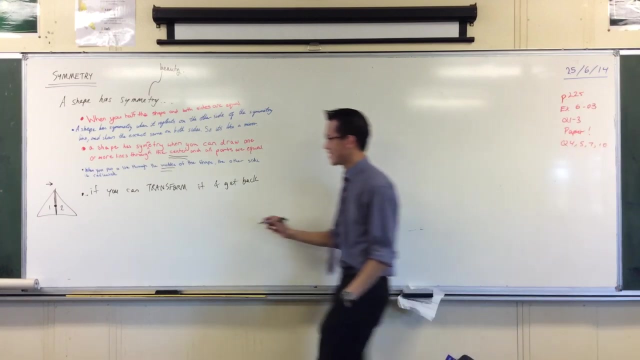 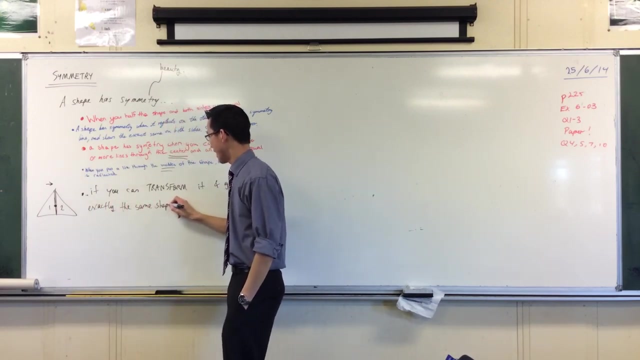 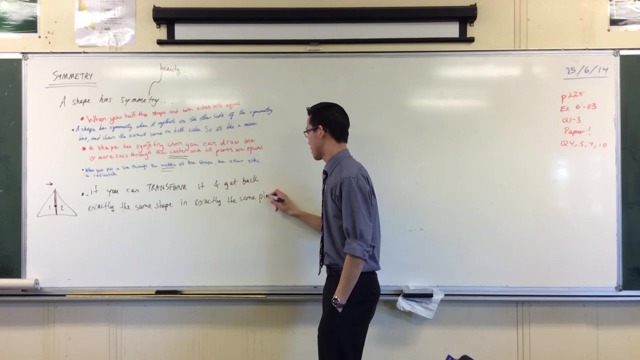 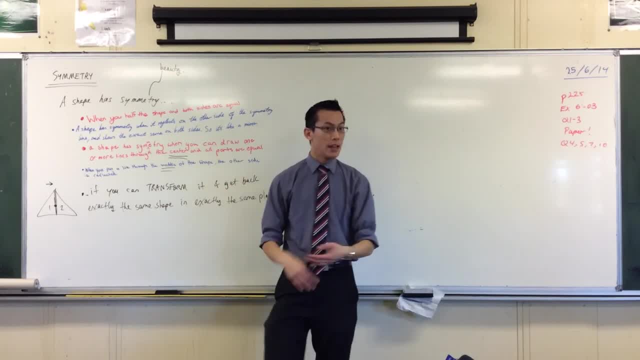 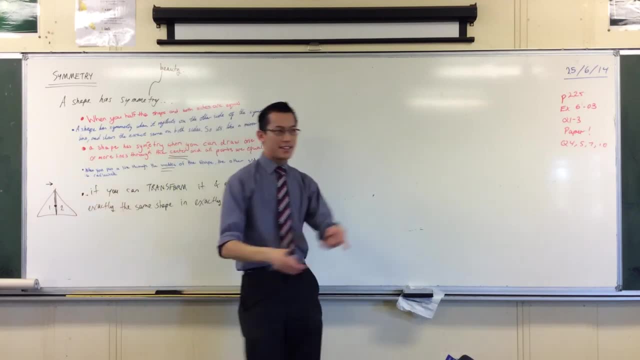 transformations are okay. so if you take one of the transformations, let's take reflection. okay, if I apply it to this shape here? right, I think there's a straight line that I can run through this so that if I apply the transformation, I just get back the same shape in the same place. that's really. 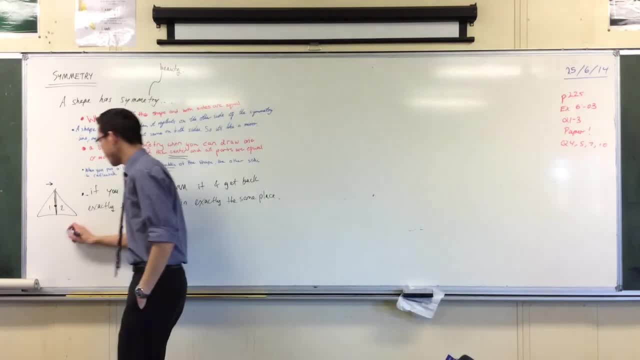 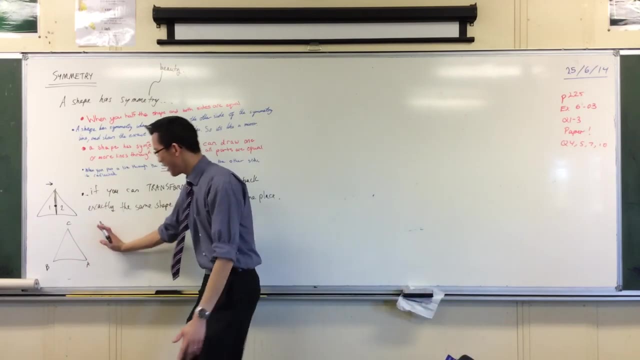 important. okay, so if I take my triangle again, right and now, the instructions I gave you were reflect this triangle. you know this would be a, B and C. okay, and I gave you a straight line now, before we look at straight lines which are like over here and over here and outside the shape, but if I draw this line through, 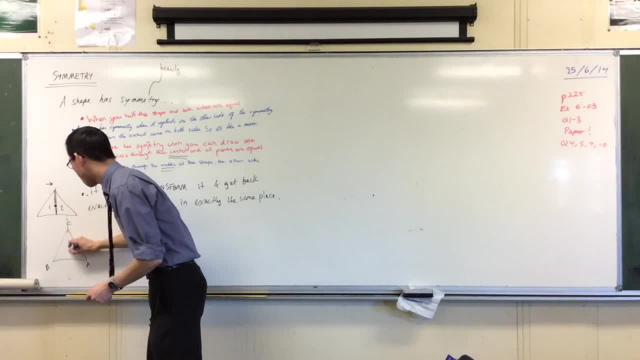 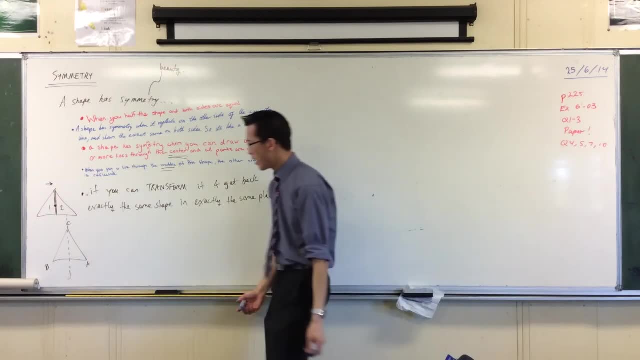 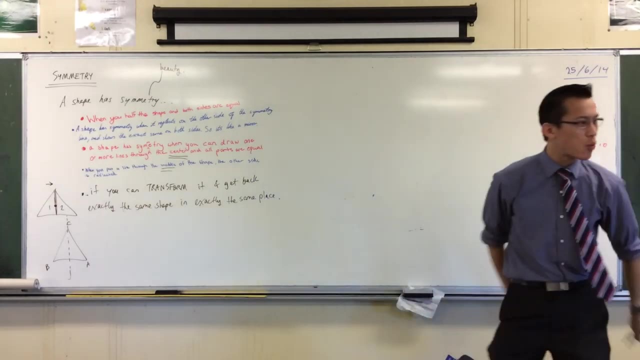 the shape just like I had before. I draw a line through like that, what will happen now? this is actually important that you draw the shape with me, because go through the process of reflection. okay, for instance, a look at a when I reflect. it's going to become a new point. before we call that a1, where will a1 be? 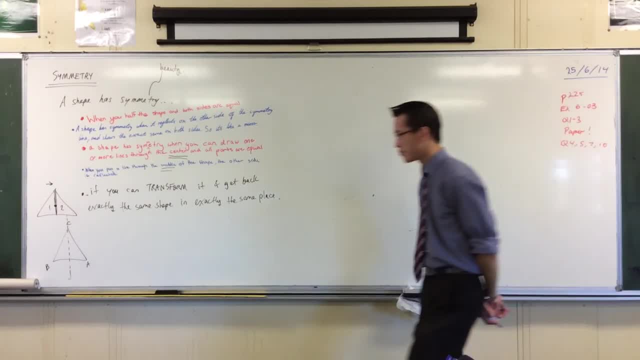 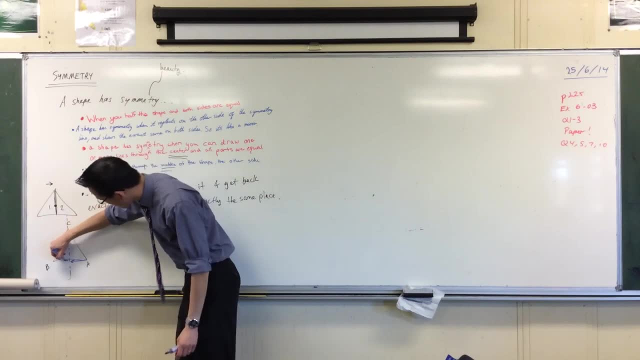 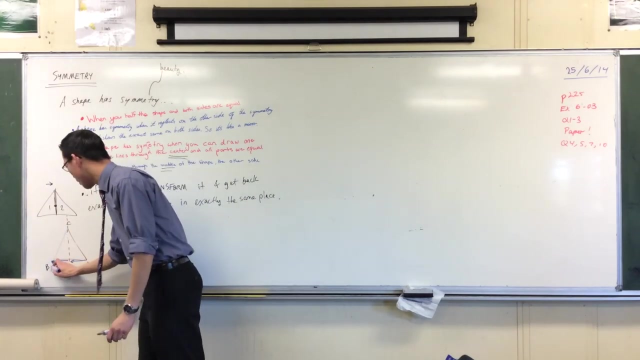 where's it gonna go if I do the same way that I do: reflection before I go this distance, right, and then I look at the opposite side of the line in the same length, right. so my new copy of a a1 is going to be over here. 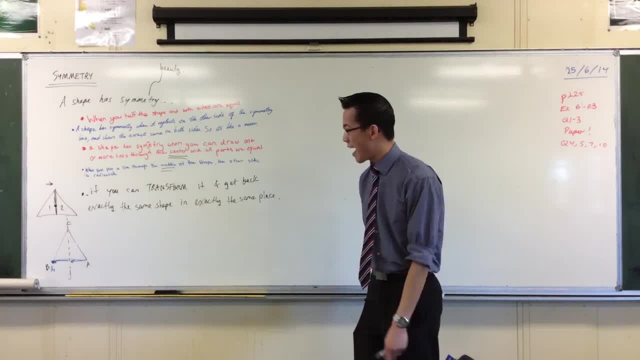 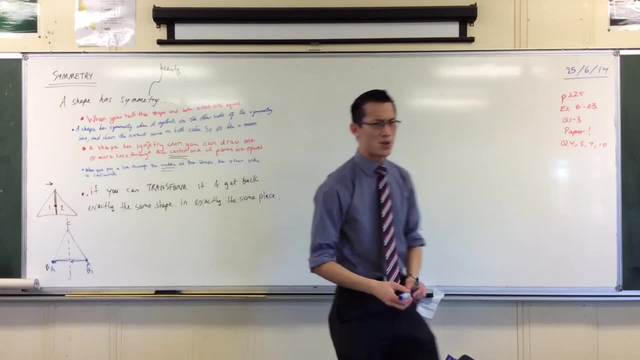 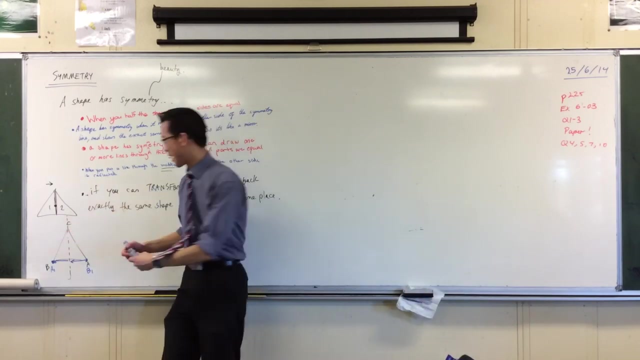 on top of B and exactly the same way, B is going to reflect across the line and become b1 over here. okay, where does he go when you reflect it? C doesn't go anywhere, right, because it's on the line of reflection. okay, so C and C one are on. 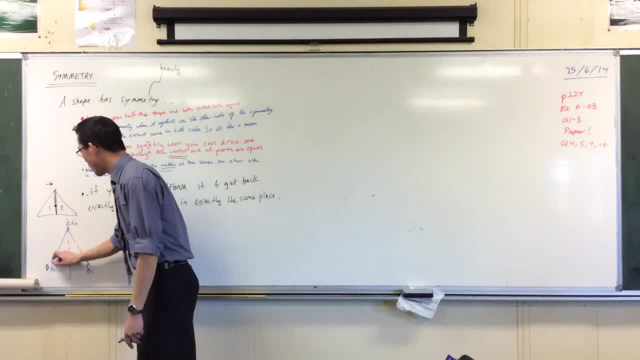 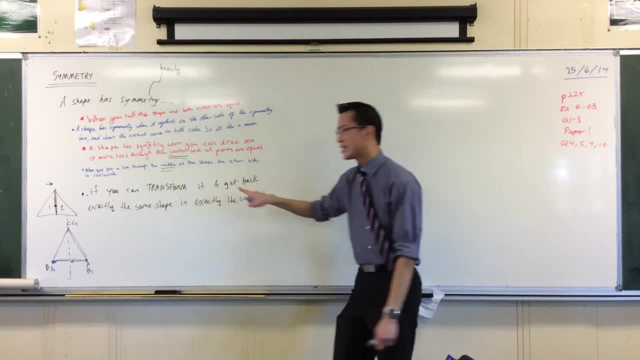 the same spot. okay, so now shape well the points. the corners are in a different order, right, they're sort of back to front this way, but it's the same shape in the same place. so we say this shape has symmetry. okay, now hold on, stay with me. I. 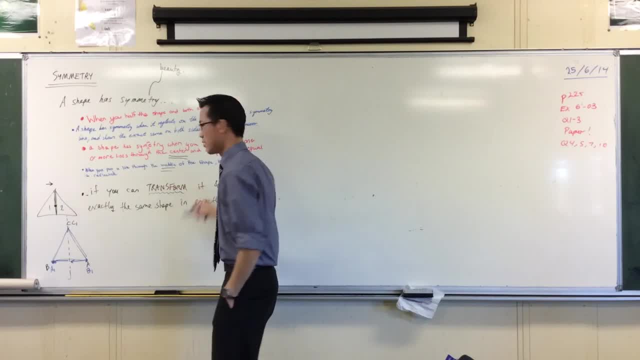 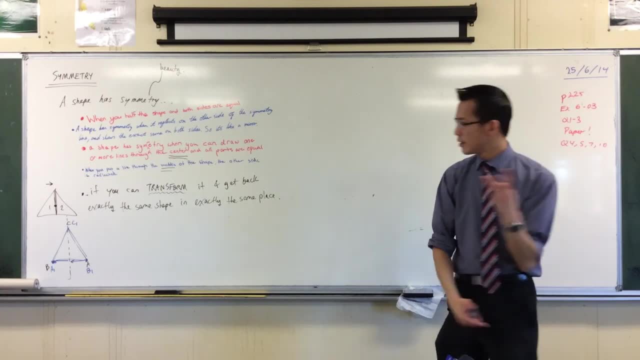 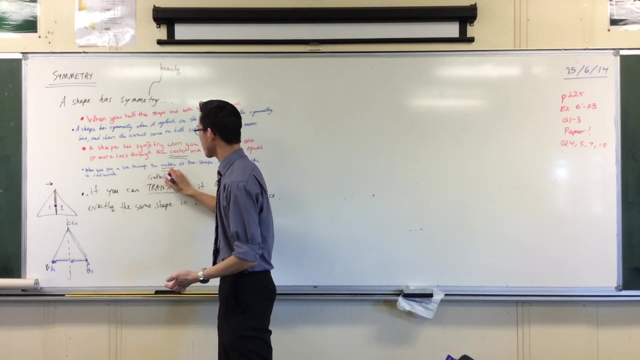 said: if you can transform it, right, but we know there is more than one kind of transformation- you already told them to me, this translation- and reflection and rotation. so this symmetry here which we've gotten from reflection is one kind: right, you can. you can reflect, but you can also rotate a shape and get a. 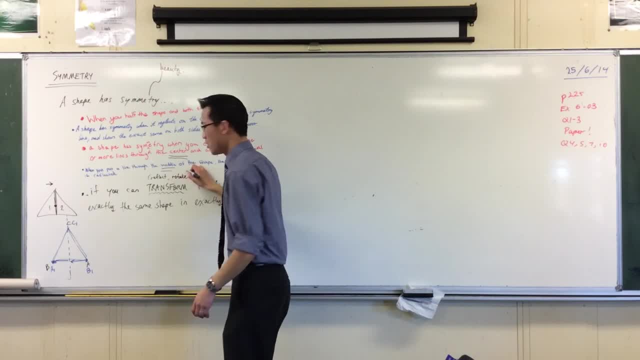 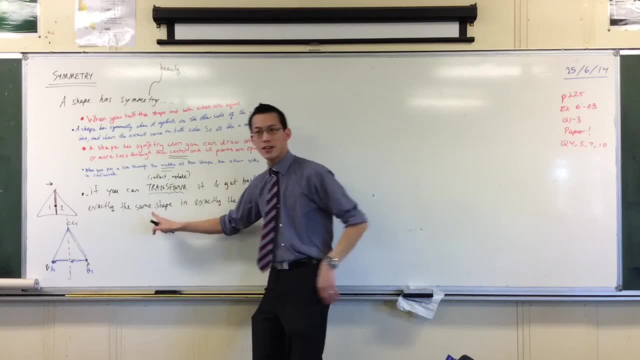 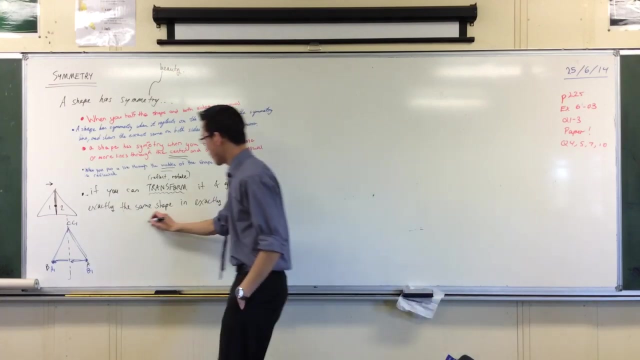 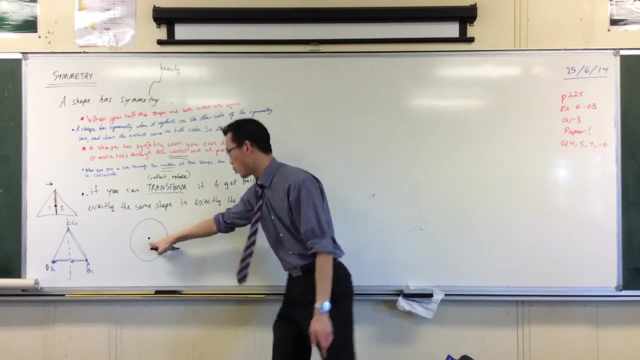 transformation, right. so, for instance, can you think of a shape so that if you rotate it in some way, you'll get back exactly the same shape in exactly the same place? hmm, yeah, a circle. great, if I draw a circle like this and I say, look, let's rotate it about the point, and I pick this point in here, right at the 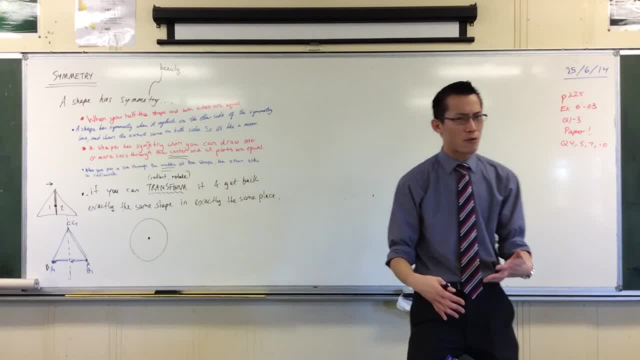 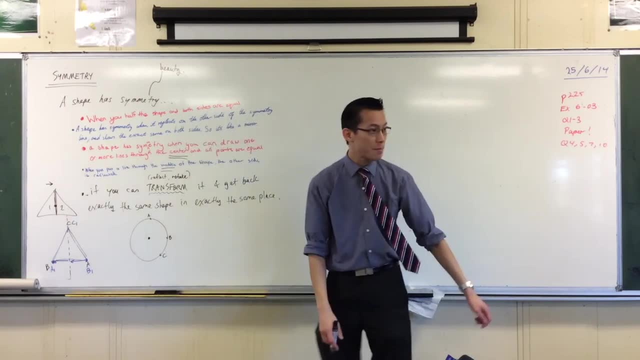 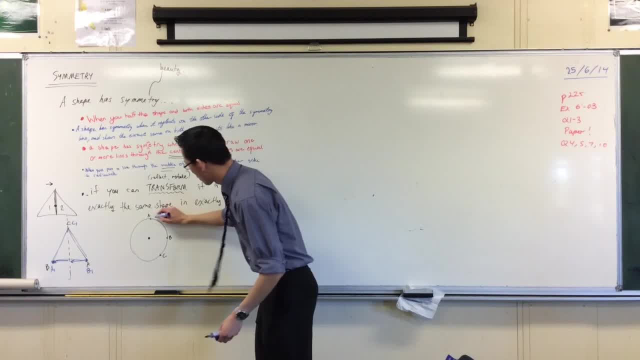 rotate it around. for instance, if I go around like this, let's go this number of degrees, however far, that is okay. so this line is gonna go there. this line is gonna go there. okay. so now I've got a: 1 and B 1 and C: 1- okay, but when I draw the 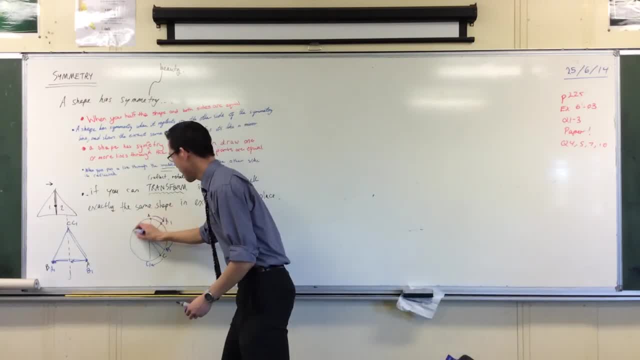 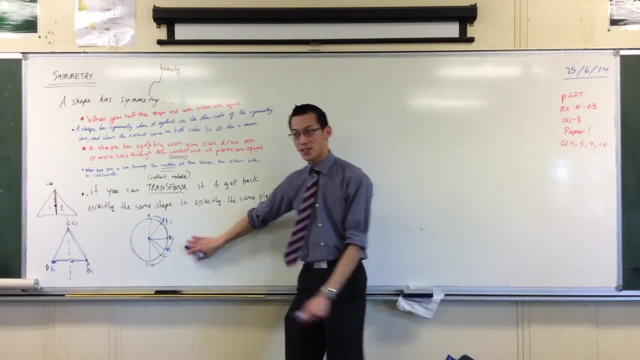 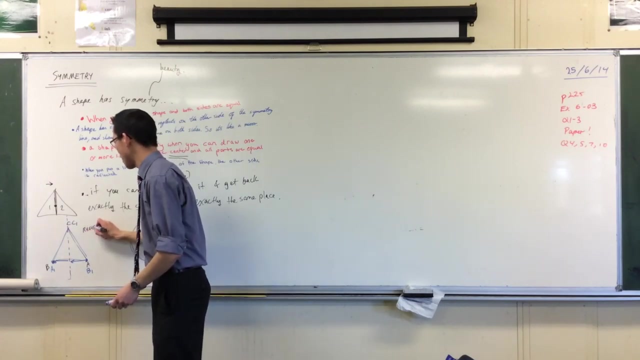 circle that goes through all these new points. it's the same circle I had before. it's the same shape in the same place. okay, now this is a kind of symmetry as well. we call this one reflectional symmetry or line symmetry. that's an important kind of phrase. you. 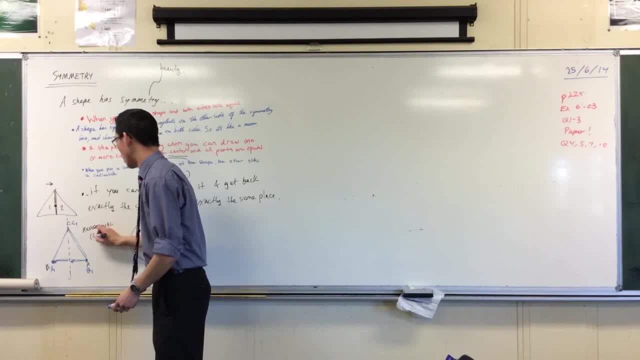 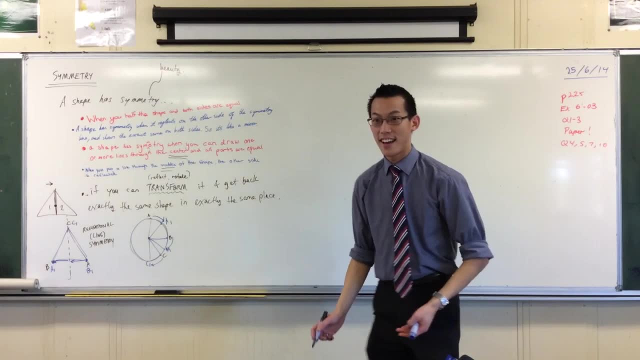 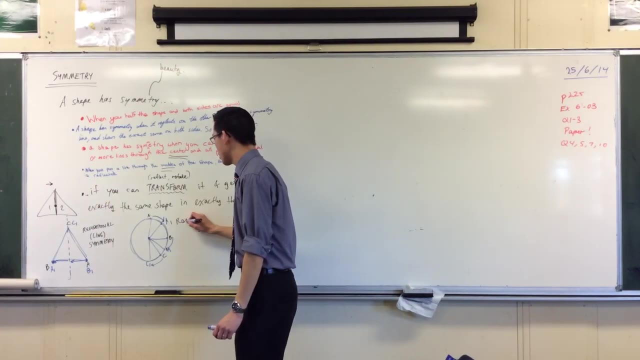 want to put that down: reflectional or line symmetry. why do you think it's called line symmetry? because when you're reflecting, yeah, yeah, the line is the piece that tells you where you do your transformation and in the same way, you do your deformation and in the same way you do your deformation and in the same way. this is called rotational symmetry. now just, 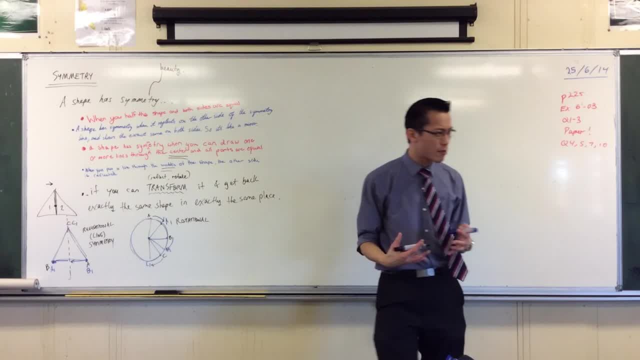 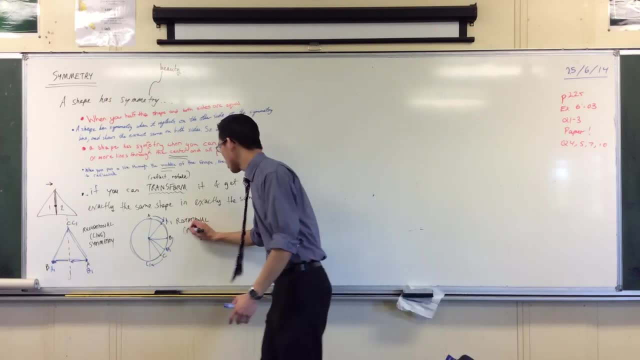 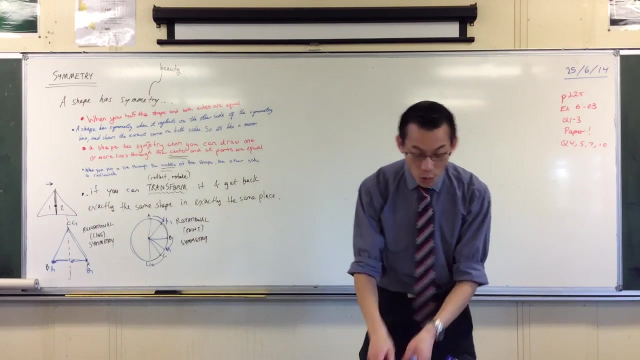 like this is line symmetry. what do you think we might call this, as well as rotational symmetry? it's not a line that we're rotating around. it's a, it's a point, so we also call this point symmetry. okay now, these kinds of symmetry are really cool. we're going to explore them in a little more depth. 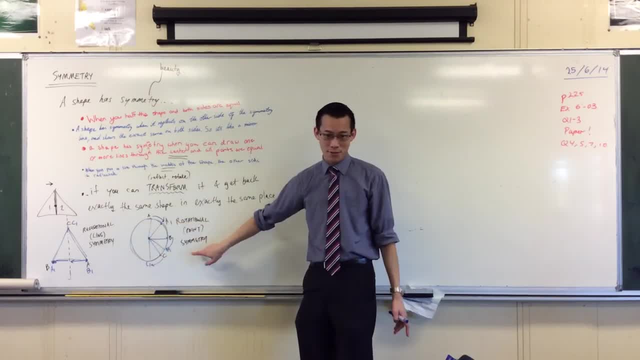 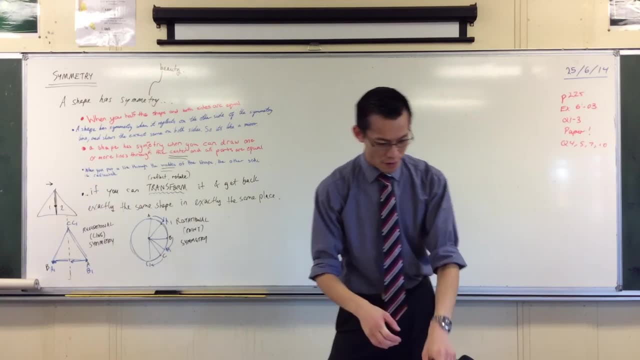 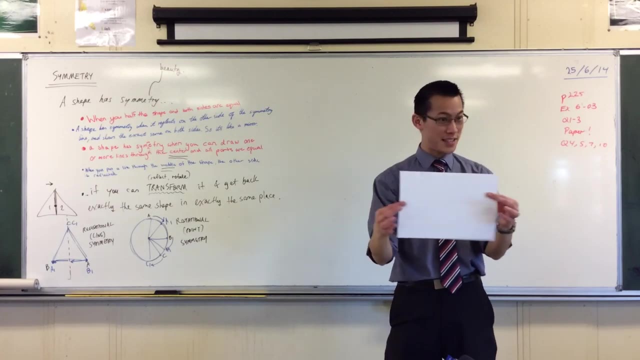 today. we're just gonna look at this one next time. we'll look at this on Friday, okay, so? So here's what we're going to do. We're going to get some pieces of paper out Now. I'm going to ask you to create some symmetrical shapes with these pieces of paper and some. 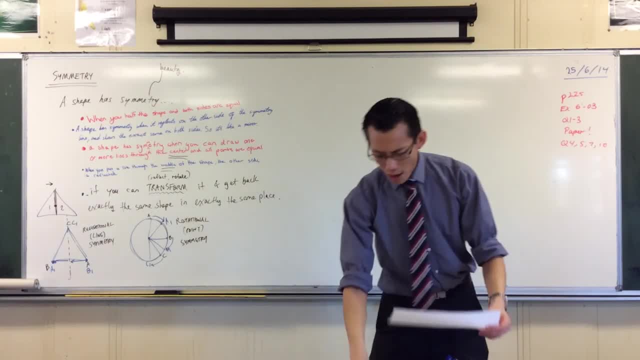 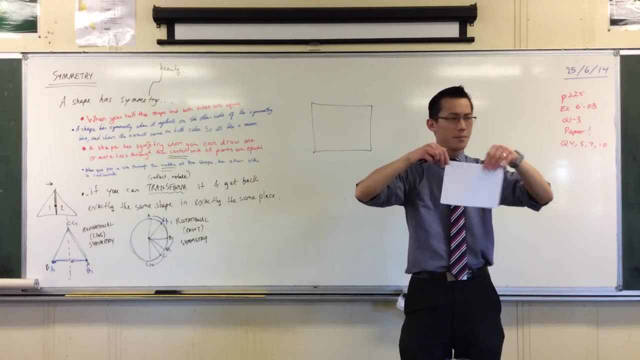 scissors. Here's the way you're going to do it On your piece of paper. now, what you're going to do is you're going to fold it. Now, this is really important. Once you fold it, there's now a line down the middle of my paper. 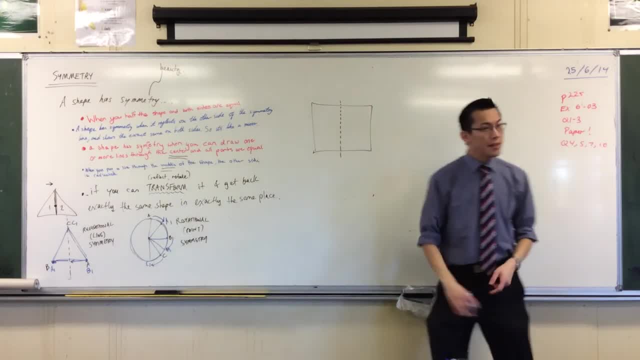 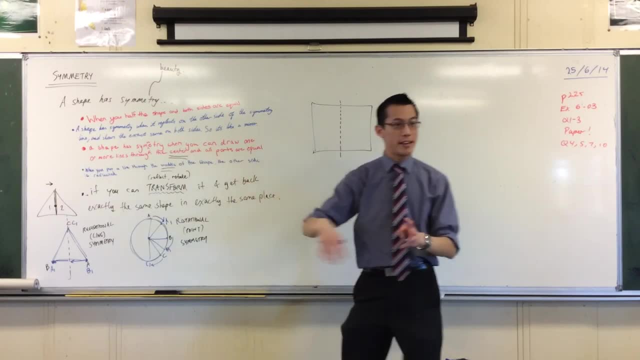 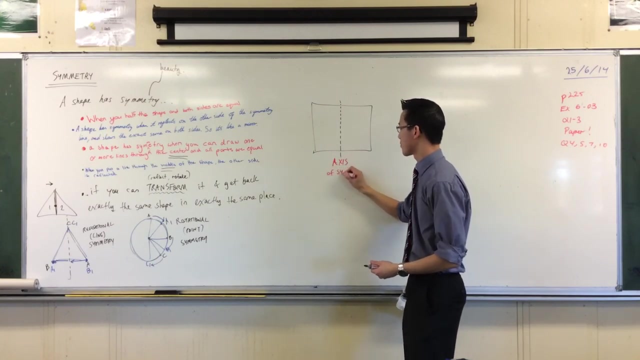 A line like this. This line is really important, This line that I'm reflecting across, that everyone's been talking about here. you know, middle centre, all that kind of thing. It's so important it gets its own name. It's called the axis of symmetry. 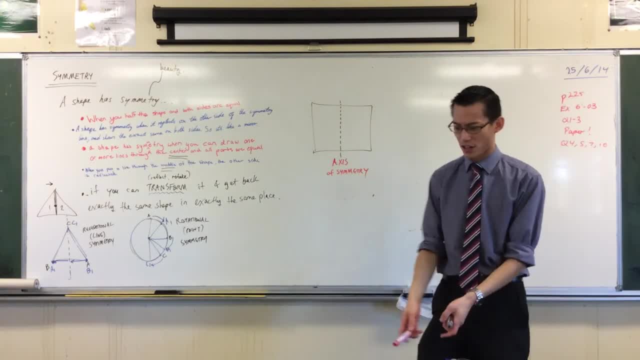 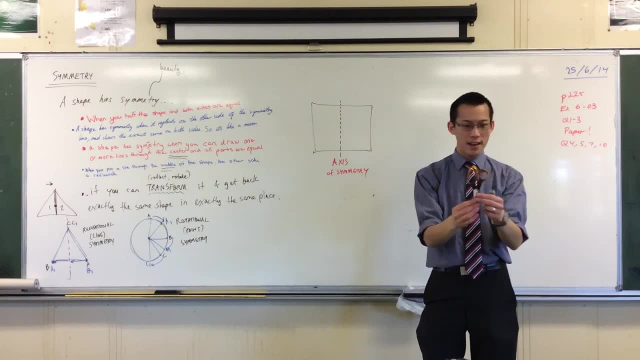 Now here's the important thing, right? Shapes. well, some shapes are not symmetrical at all. right, Here's my pair of scissors. My pair of scissors is not symmetrical. There is no line that you can draw. You can draw through it such that, if you reflect it, you get the same shape in the same place. 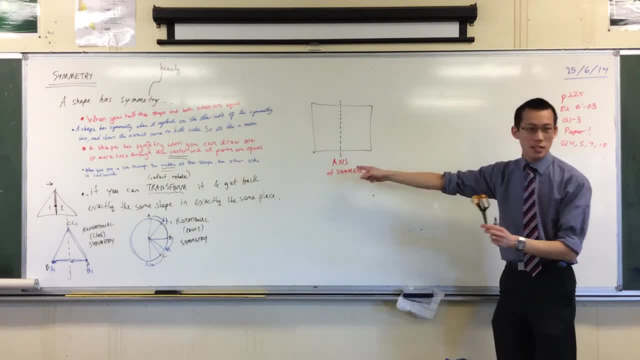 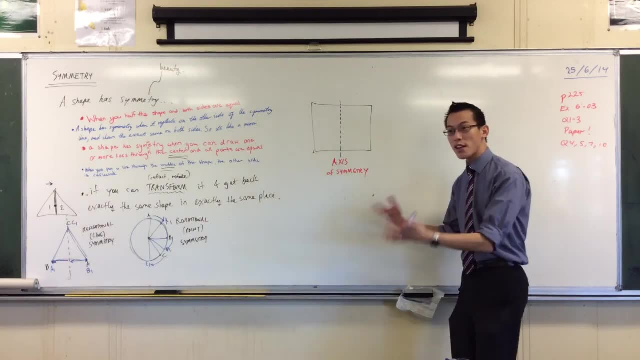 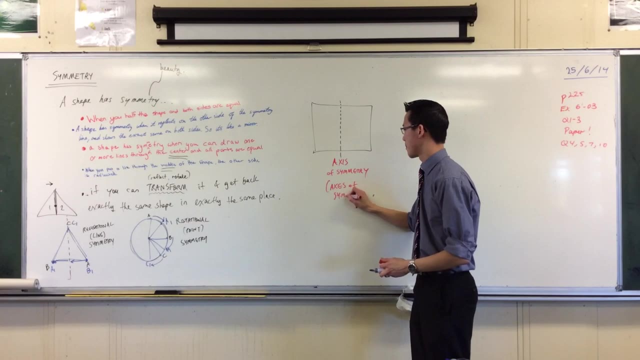 So some shapes have no axis of symmetry. Some shapes have one axis of symmetry, okay, And still others will have lots of different- and there's a plural word- lots of different axes of symmetry, Okay, So get this axis: axis, that's the singular. 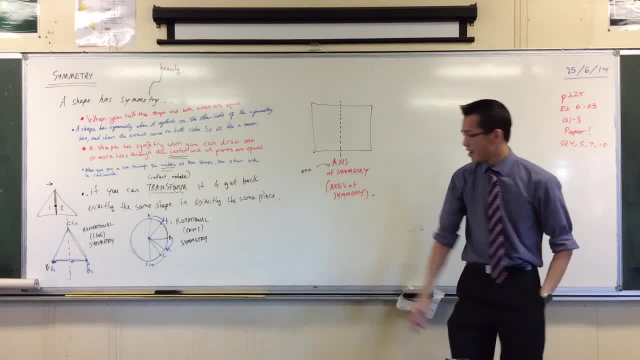 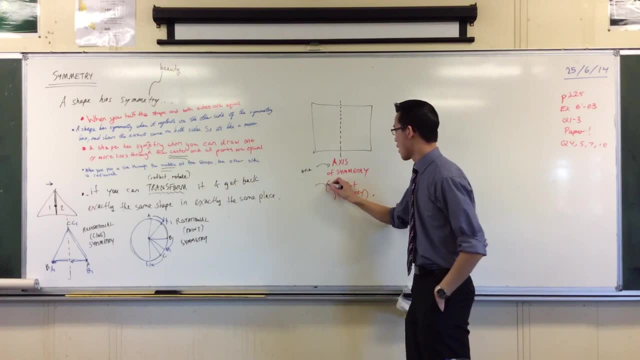 That's when you've just got one, Okay, You can have one axis. but if you've got lots, if you can draw lots of different lines and reflect across and get the same shape in the same place, you have many axes of symmetry. 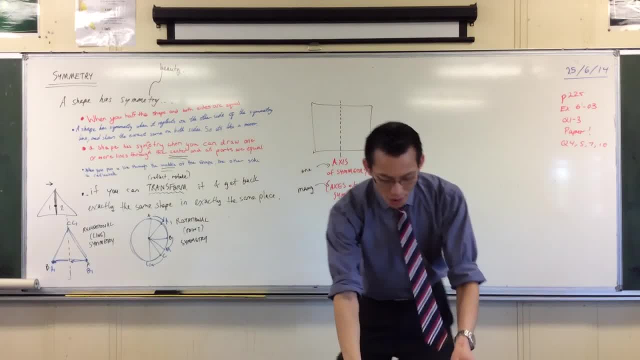 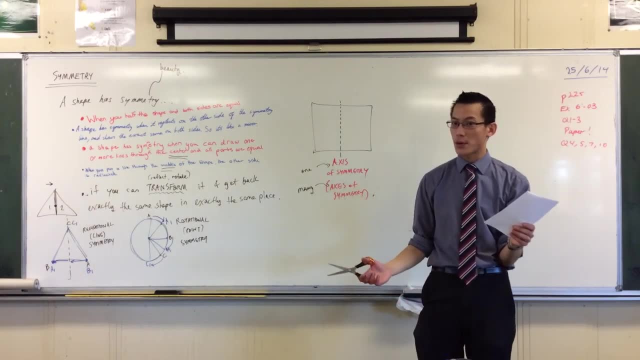 Okay, Singular plural. Now, once you do that, okay, you're going to draw your cut your line across here, sorry, fold your line, okay. And then I want you to cut a shape, okay. Now, here's the cool thing. 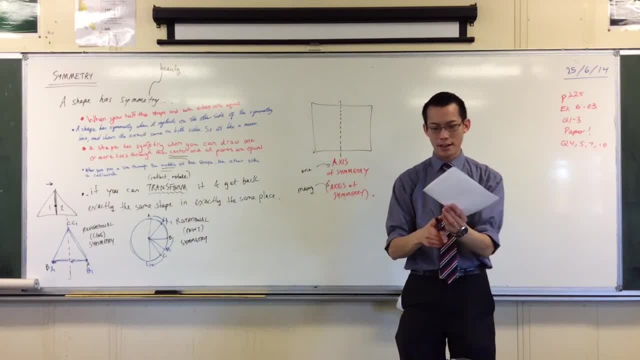 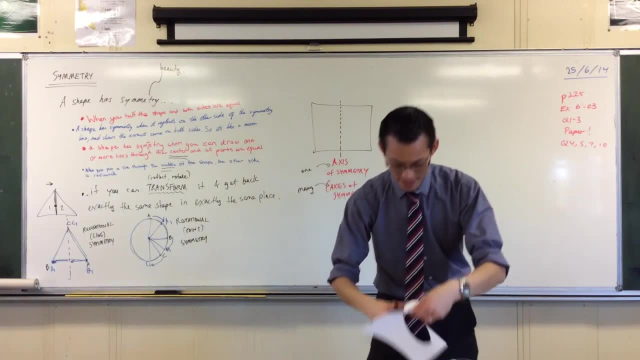 If you cut across this line any shape you like, okay, For instance, I might cut this. Let's see if I can do this. here we go. Okay, so I've cut a shape out, right, But when I unfold it, I should get a symmetrical shape. 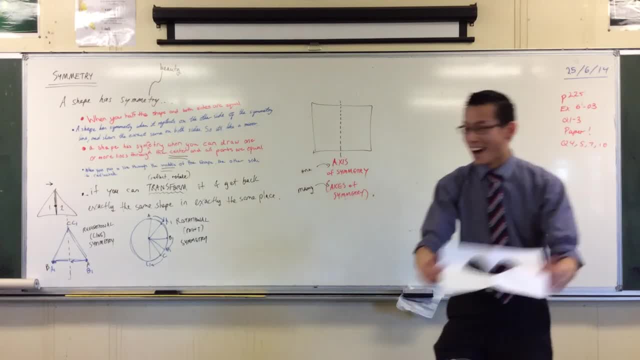 Thank you, Mr Poole. Okay, Oh, you're welcome, Mark, It wasn't for you. Now, what you've got there is a symmetrical shape. okay, We're going to do this a couple of times for everyone. 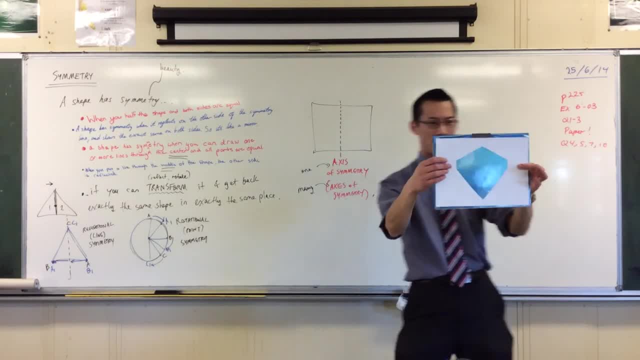 You can do some interesting shapes right. Here's one, There you go. You can see that right, And you can see there's the axis of symmetry. Okay, But you can do an interesting thing. That's a bit boring. 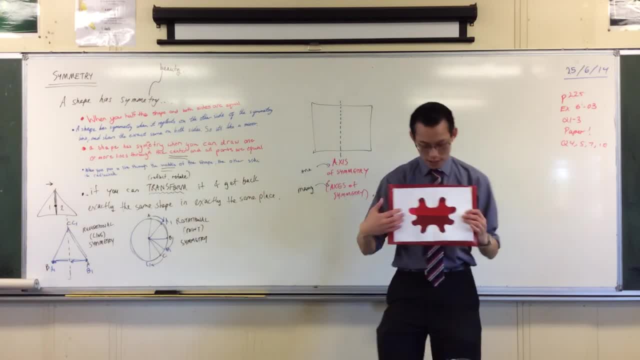 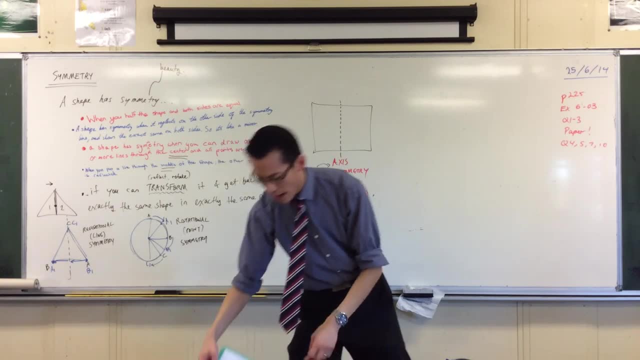 That's a bit straight. You could do something like this: This is still symmetrical and you can just barely see the folds, right. You can even do some shapes that are disconnected, okay. So you can see if I do it this way, okay. 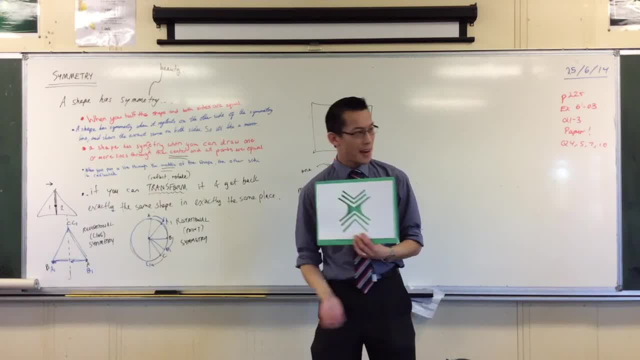 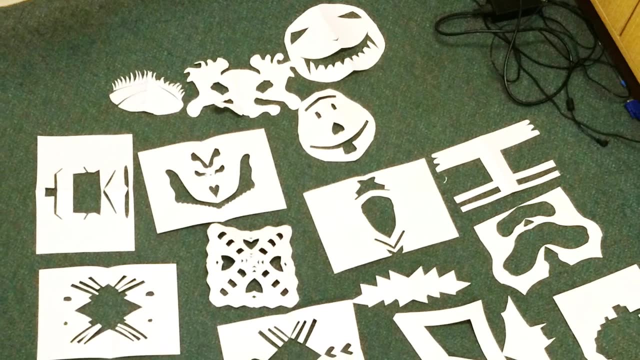 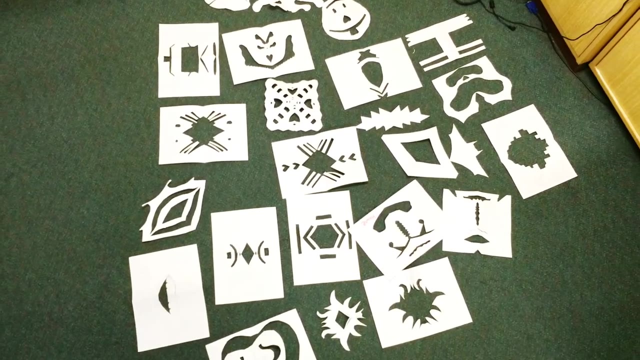 There's the axis of symmetry, depending on what you cut. okay, So here's the way we're going to do it. So what we're going to do is we're going to cut this. See, We're going to cut this. See, See, I know, I know I'm going to cut this right here, So we're going to do that. This is just for the camera. It's a lot easier than I thought. It's a lot easier than I thought. Yeah, I like that. There you go, I like that. Okay, Awesome.